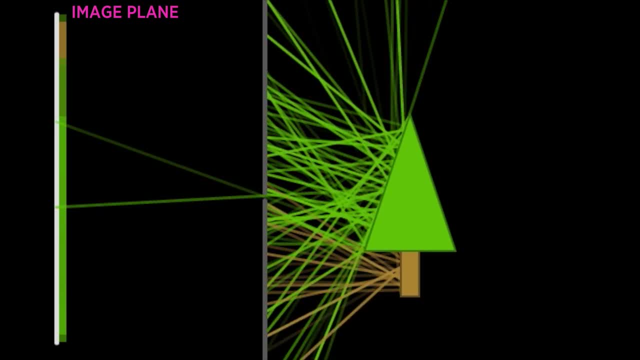 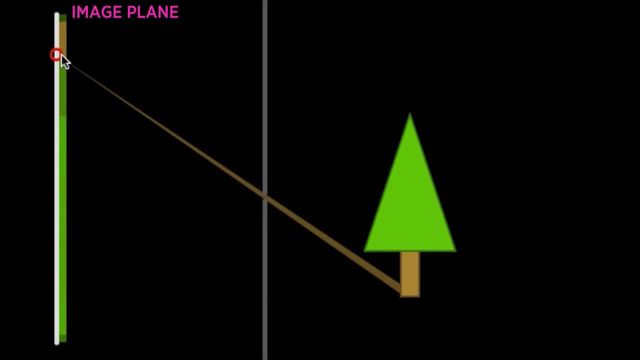 aperture only lets certain light rays through. At this point here on the image plane only light rays from one direction can make it through the aperture, And those light rays come from light bouncing off this place in the scene. So the aperture is filtering out any light rays. 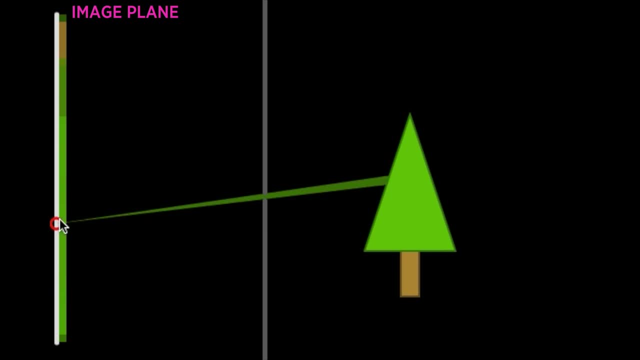 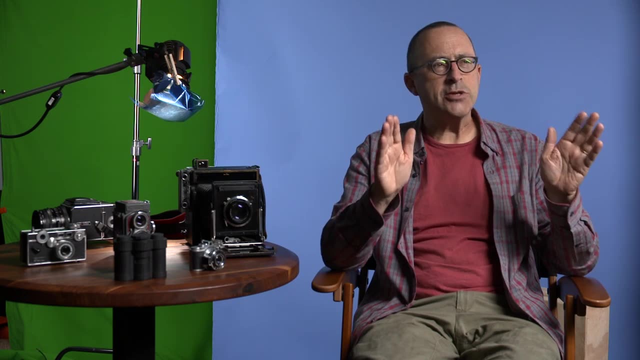 that don't come from the right direction. This simple camera design is known as a pinhole camera. If we replaced the back wall of the room with a great big sheet of photographic film, we could take a great picture that way. Did you know that the word camera 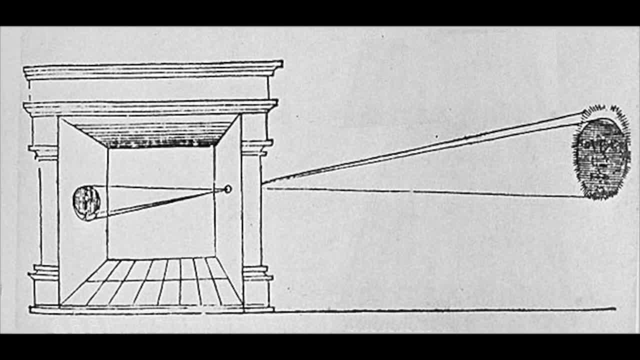 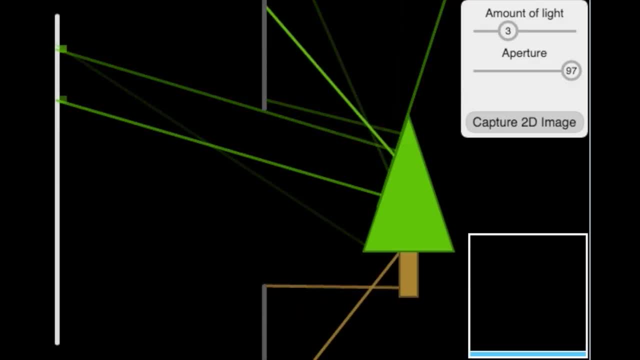 comes from the Latin word for room. The first cameras were known as camera obscura, meaning darkened room. They were, in fact, room size like our office. In the next exercise, you can use this pinhole simulator to take some virtual pictures. 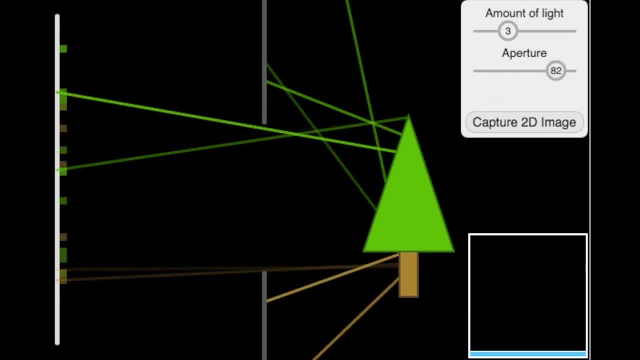 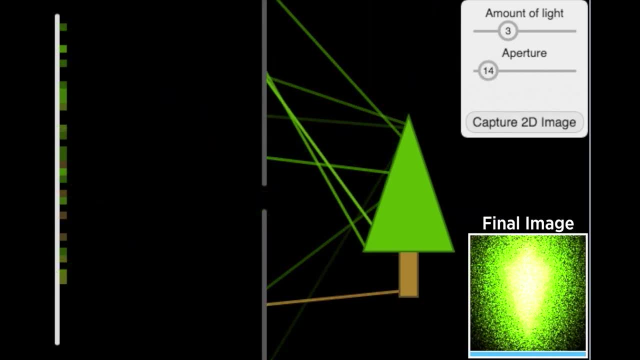 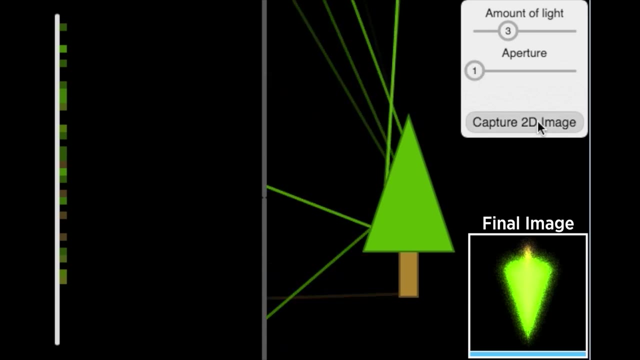 You can adjust the size of your pinhole or aperture and press here to capture an image. While doing so, you'll have to answer some questions about what's going on, such as why is the image flipped and, more importantly, what happens if we change the size of our aperture. See you in a moment. 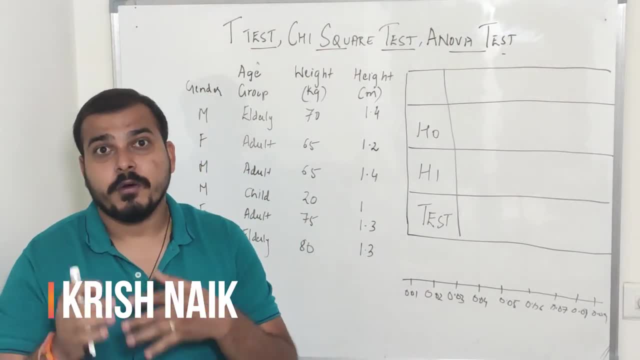 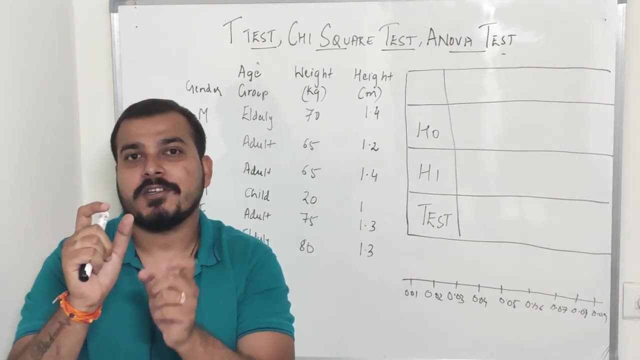 Hello all my name is Krishna and welcome to my YouTube channel. Today, in this particular video, we will be discussing about t-test, chi-square test, ANOVA test, and we will also be discussing about a very important thing which is called as p-value, which is also called as significance value. 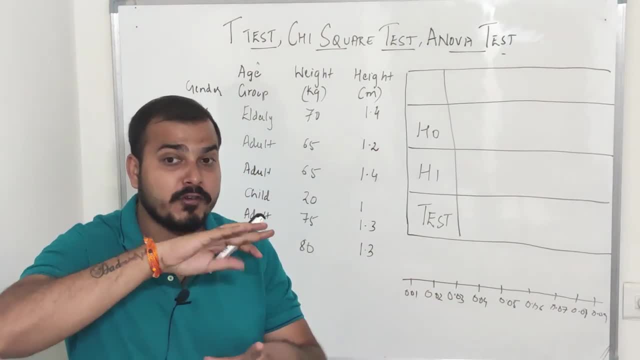 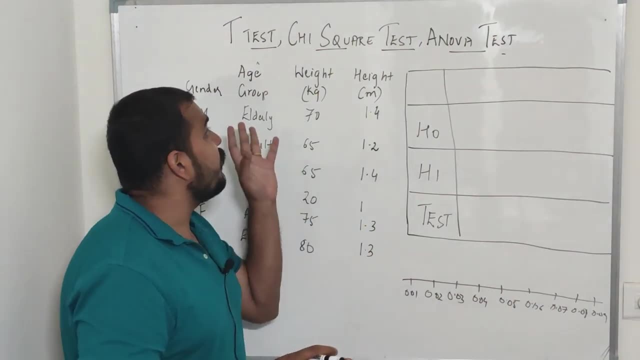 Now, guys, in my previous video, I have already explained you about hypothesis testing and I gave you your overall overview about it. We have discussed about null hypothesis, alternate hypothesis, But now, in this particular video, we will focus on when to use t-test, when to use chi-square test, when to use ANOVA test. 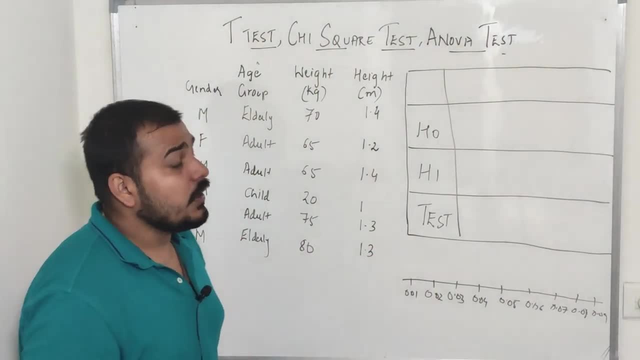 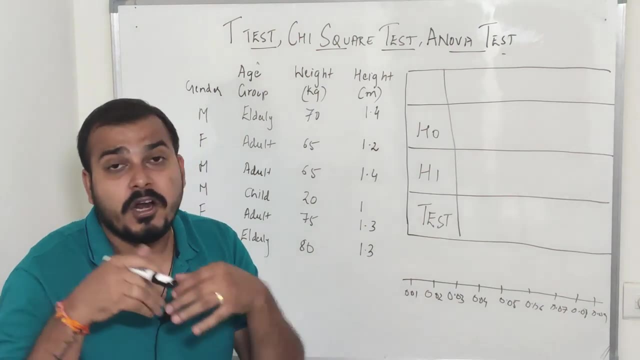 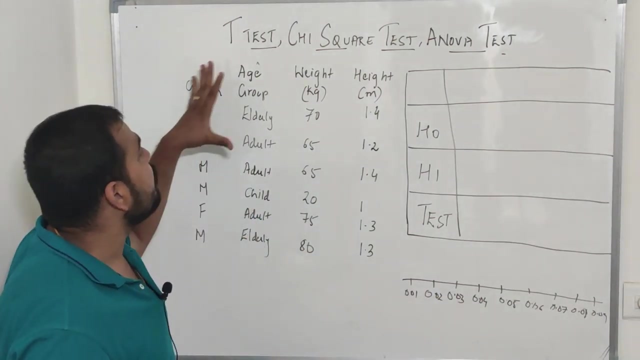 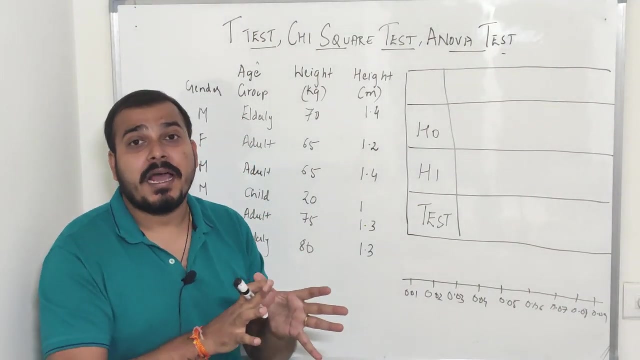 We are going to discuss about this. So, guys, and one more confusion that I usually get from students and some of my subscribers is that they are not able to relate this concept to the real world scenario. This is the main problem over here. So I am going to take a very simple data set over here and remember, guys, this is a sample of the data set and, as you remember, I told you that when we are discussing about hypothesis testing, we come to a conclusion for a population based on a sample data set.